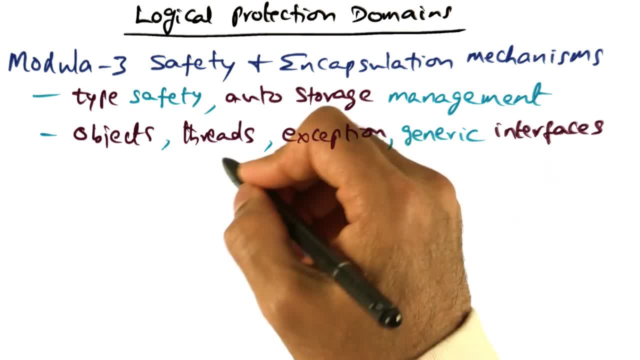 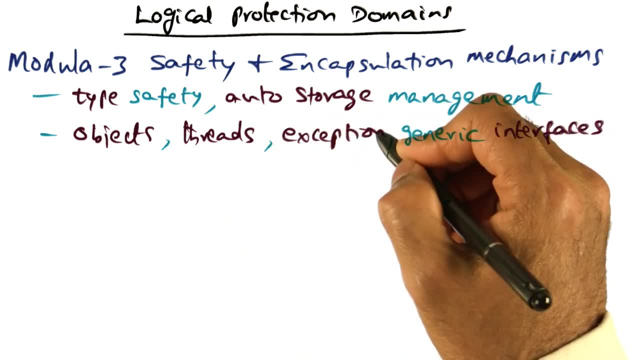 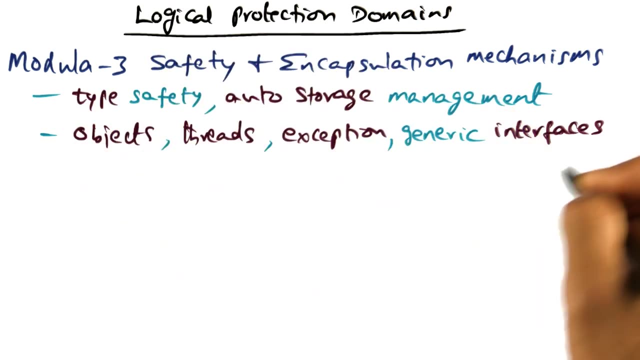 using generic interfaces, And it also supports the notion of threads that execute in the context of the object And it allows raising exceptions, for example when there is a memory access violation. All of the features that I mentioned here in a nutshell allows implementing system services. 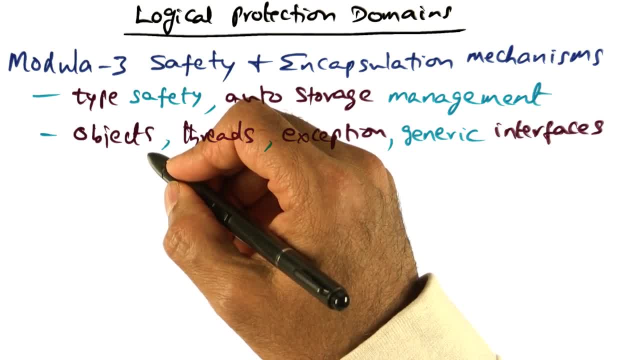 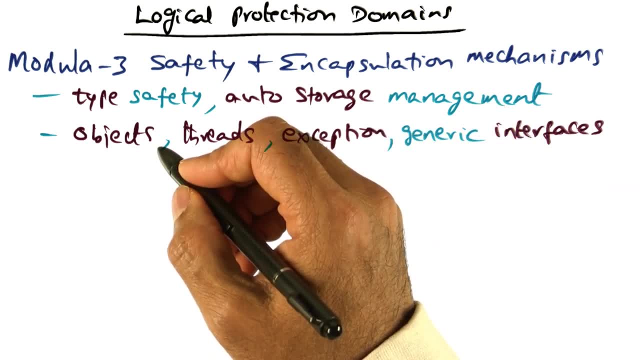 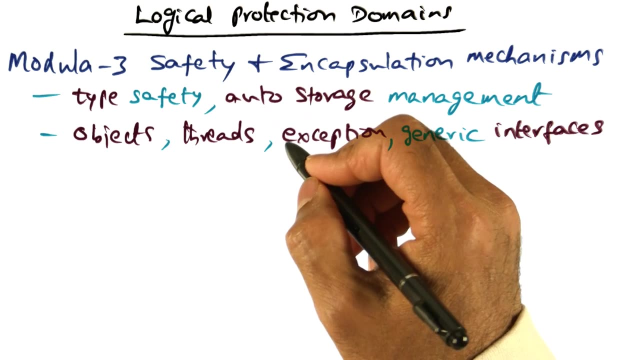 as an object with well-defined entry points. This modular 3 allows the creation of logical protection domains. What you can do from outside the object is what the entry point methods that are inside the object will let you do, and no more. In other words, 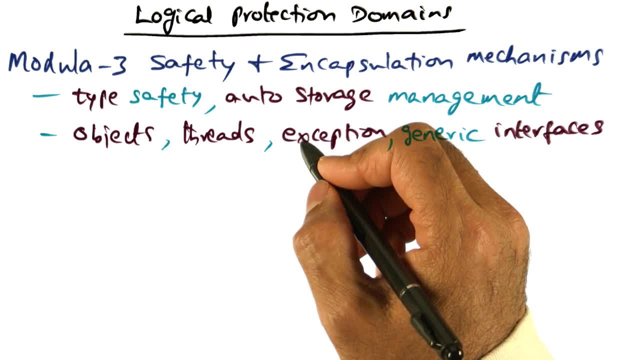 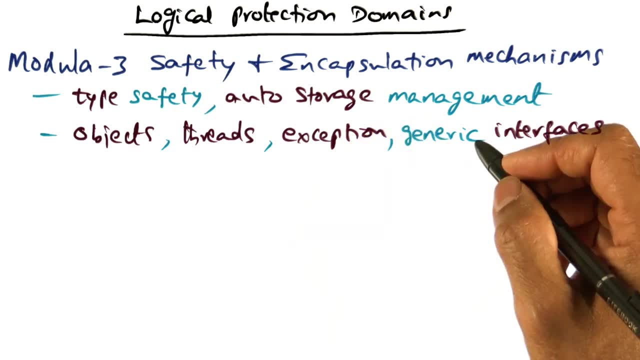 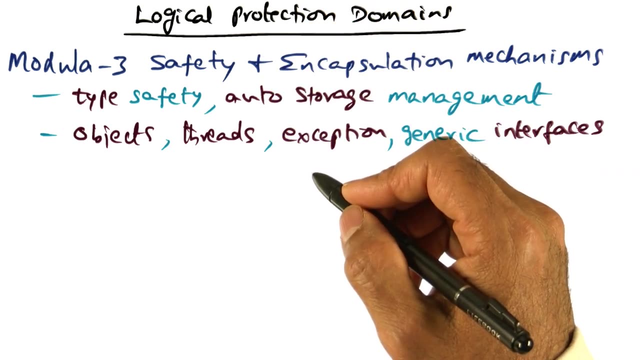 we are getting the safety property of a monolithic kernel without having to put system code in a separate hardware address space. So, in other words, the logical protection domains give you both protection and performance, the two things that we strive for Now. what about flexibility? 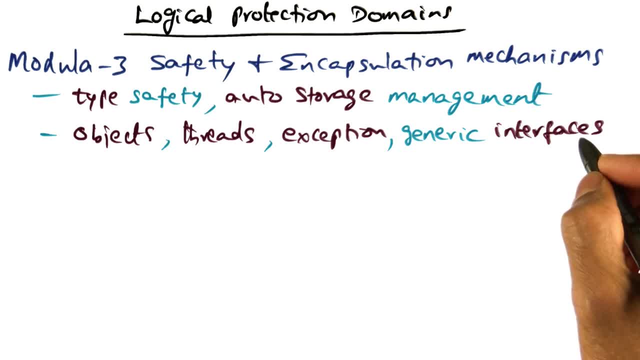 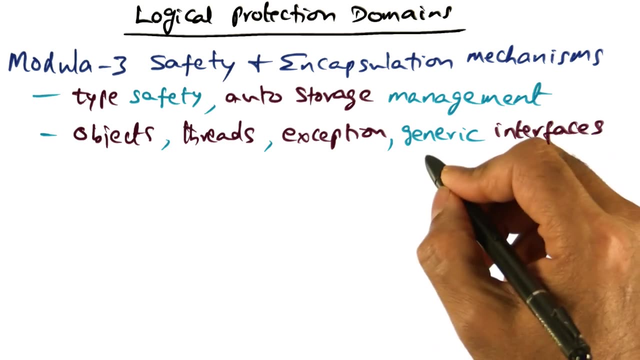 Well, the generic interface mechanism allows you to have multiple instances of the same service, And a given application may be able to exploit the different instances of services that are available that cater to the same generic interface, and that's the way you can get flexibility as well. 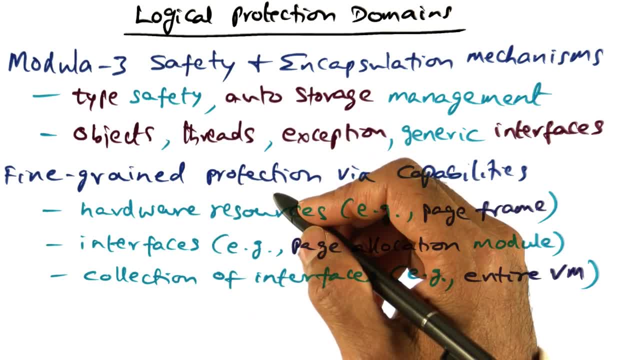 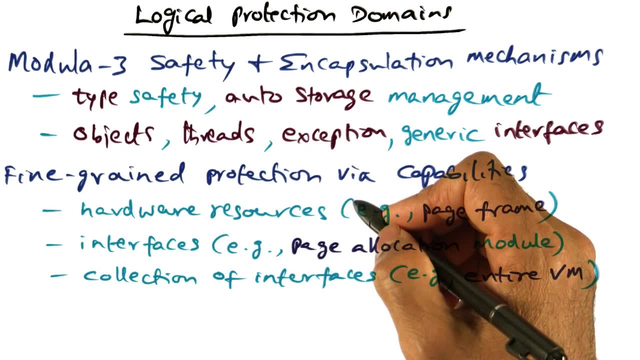 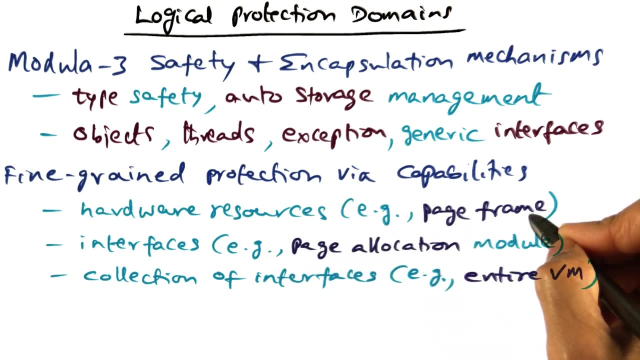 And objects that implement specific services can be at the desired granularity of the system designer. It can be fine-grained or it can be a collection. You can think of individual hardware resources as fine-grained object, for example a page frame and what you can do with a particular page frame. 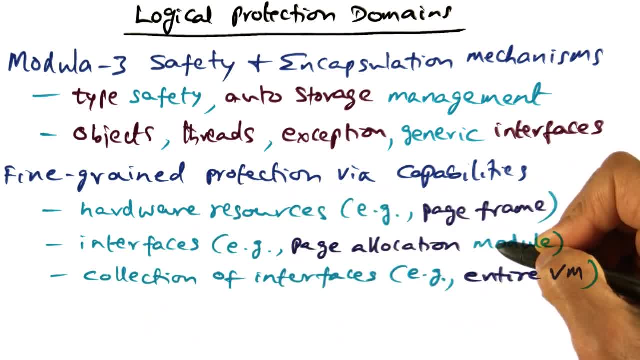 You can have interfaces that provide a certain functionality. That can be what an object is. For example, a page allocation module can be an object, And you can also make a collection of interfaces into an object. For example, an entire virtual memory subsystem can be an object that is hierarchically composed of page.